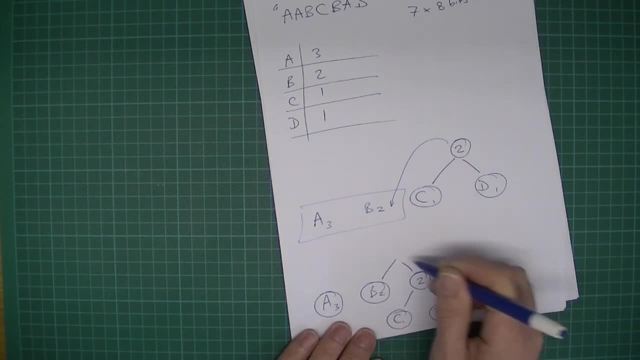 there's 2.. Add them together: 2 plus 2 is 4.. And then- remember, this is priority queue- This 4 is greater than 3, so when we rewrite it, we're going to put it that So this time around. 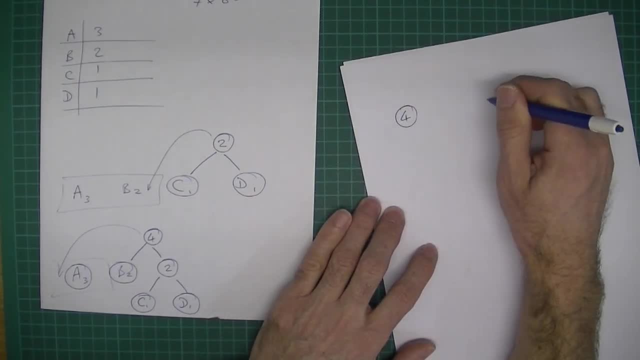 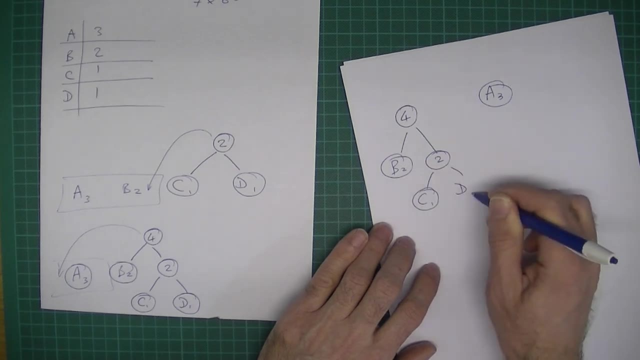 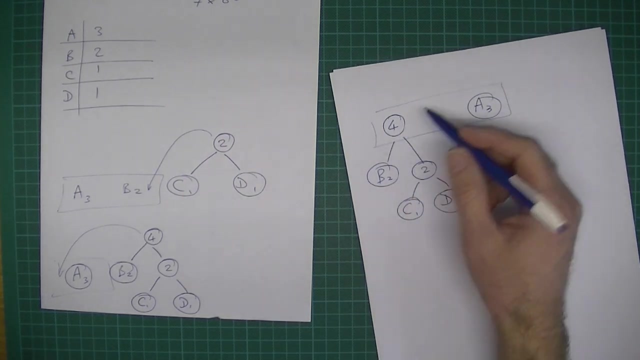 We've got 4 here. We've got A with a frequency of 3 and a frequency of 1.. That's now our new priority queue And we need to join these 2.. So 4 plus 3 is 7.. And now that's our new. 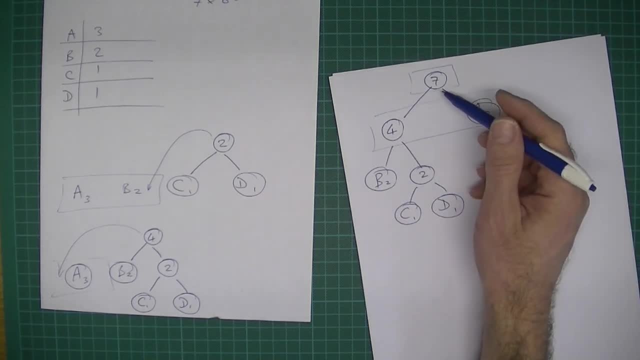 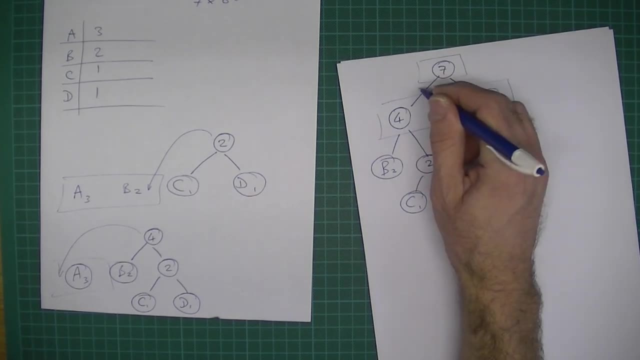 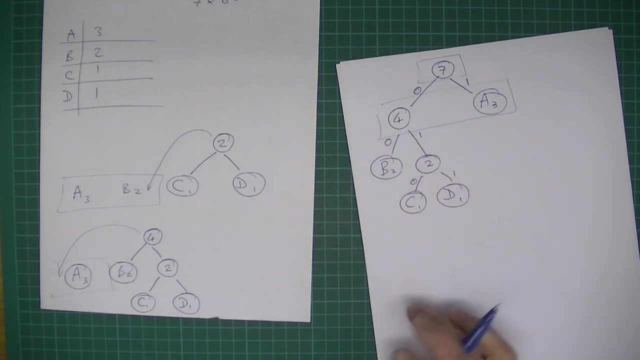 priority queue. There's only one item in the priority queue, so our algorithm says: stop at this point. Now, this is a Huffman tree. And now on the left, by convention, on the left hand side, it's going to be binary bit 0.. Right, it's going to be 1.. And now, going back to this frequency, 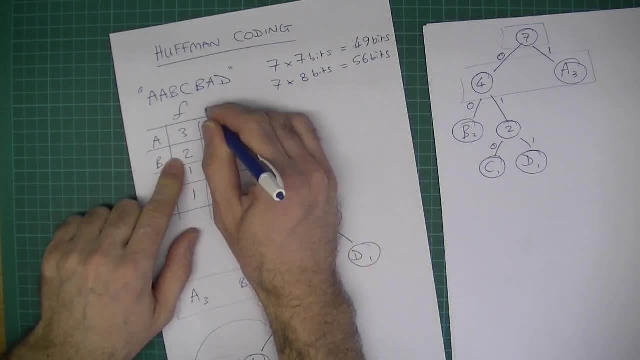 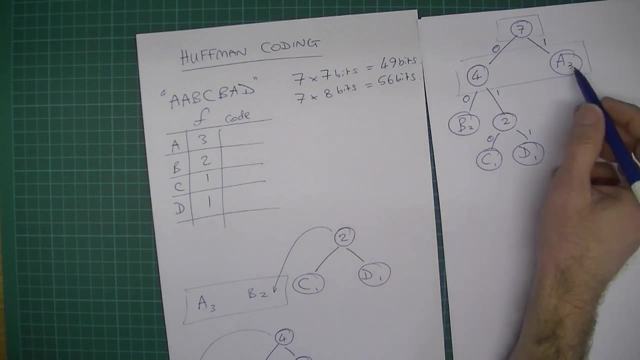 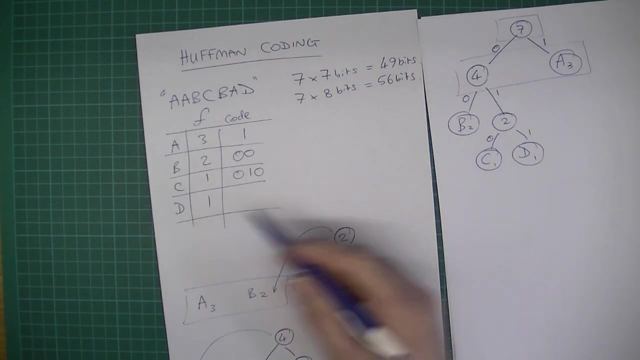 table. So those are the frequencies, and then we can write the Huffman codes here. So let's take the letter A to start with. Well, The letter A is just 1.. The code for letter B is going to be 0, 0.. 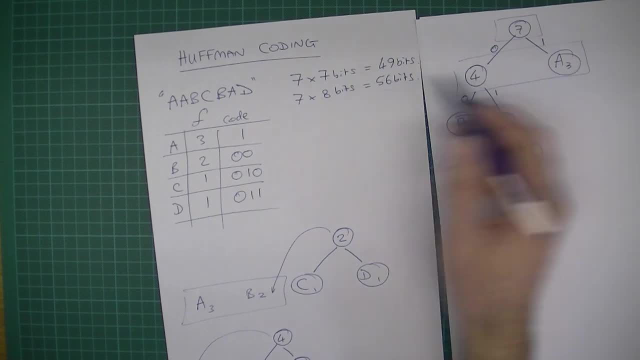 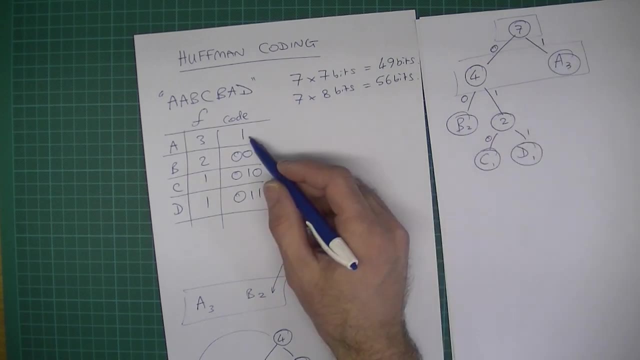 What you might notice is the most frequently occurring letter, which in this case was letter A, because that frequency of 3, which is greater than the other ones, is going to have a nice short code, And that's important. So now that we know the codes, we can encode this, So we'll 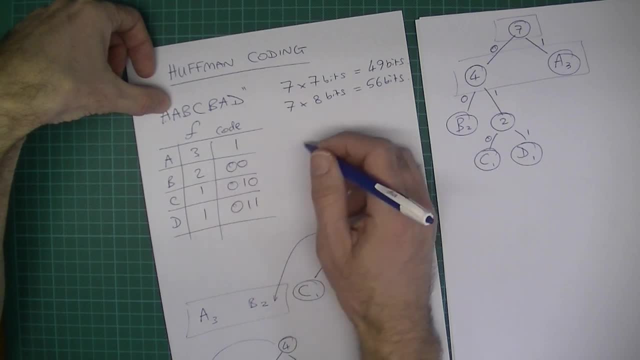 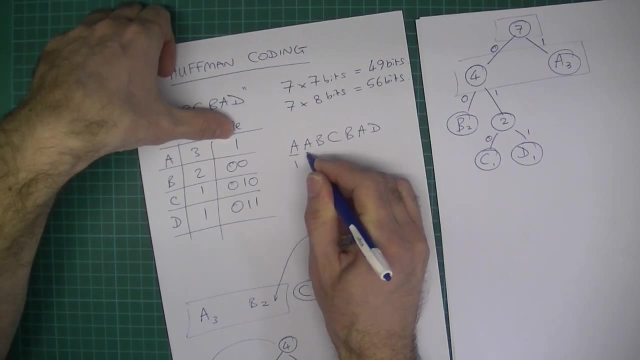 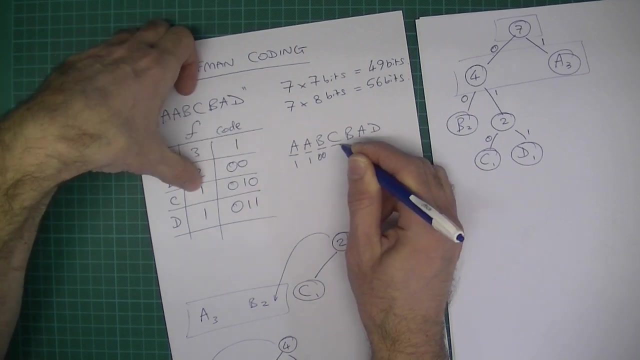 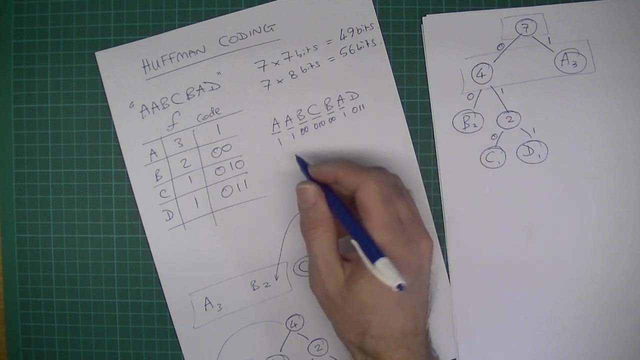 encode this. So letter A is 1.. So let's just rewrite this. So the letter A is 1.. The letter A is 1.. The letter B is going to be 0: 0.. In Huffman coded bit patterns there won't be any spaces, So let's just write it out.